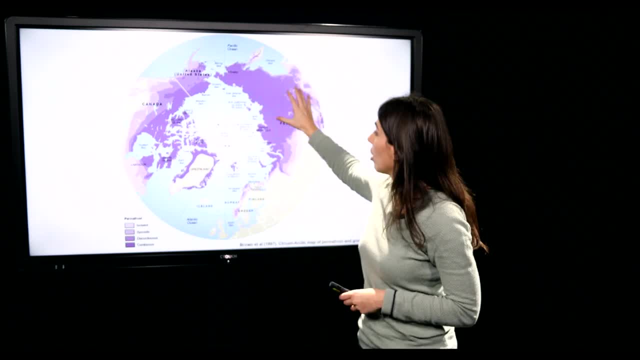 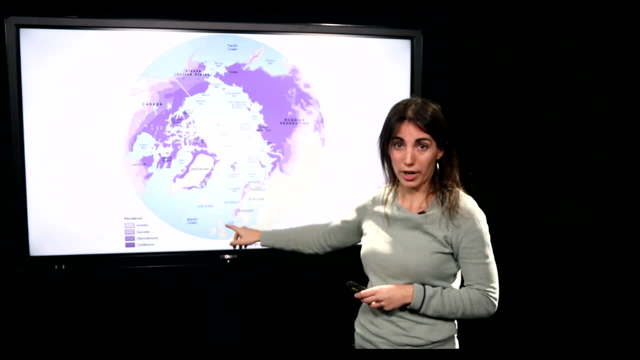 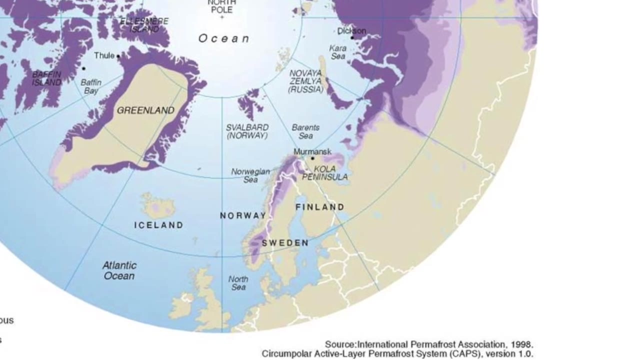 with the purple areas. So we can see here that large areas of Russia and Canada have big areas of permafrost. but also in Norway we have areas with permafrost And that prevents releases from carbon. So what happens when permafrost thaws? 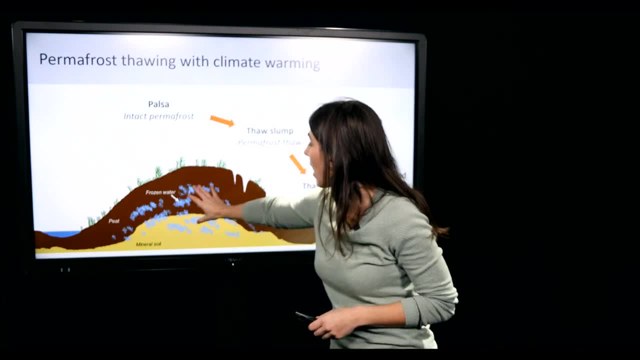 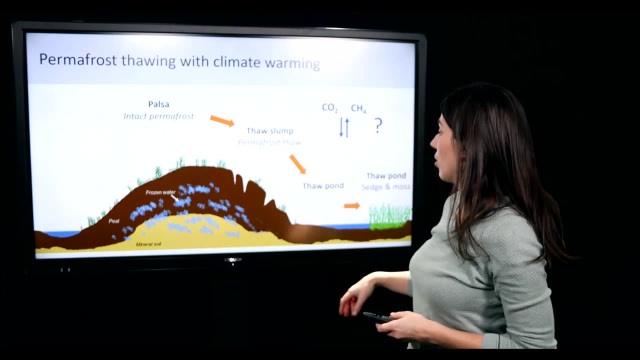 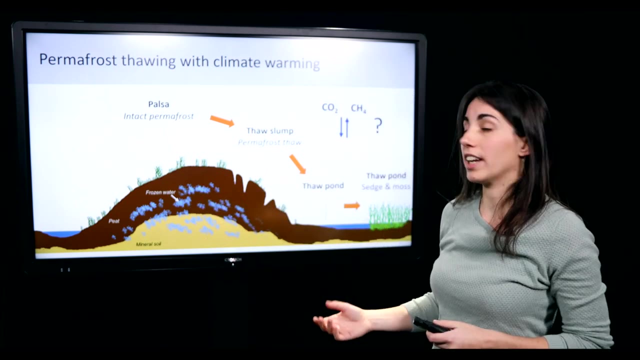 We have here a picture of permafrost that is intact where the soil is frozen and when it starts to warm, permafrost starts to thaw. This means that the frozen water in the soil is melting and this is causing the permafrost to thaw. 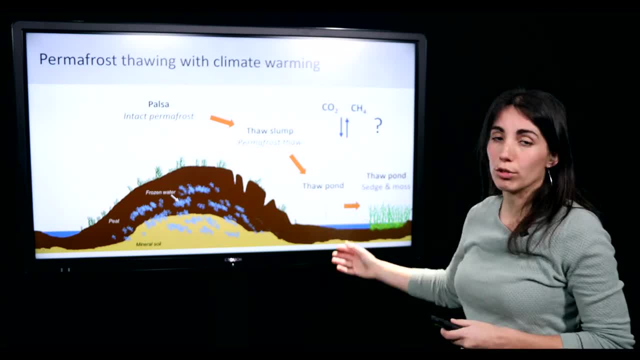 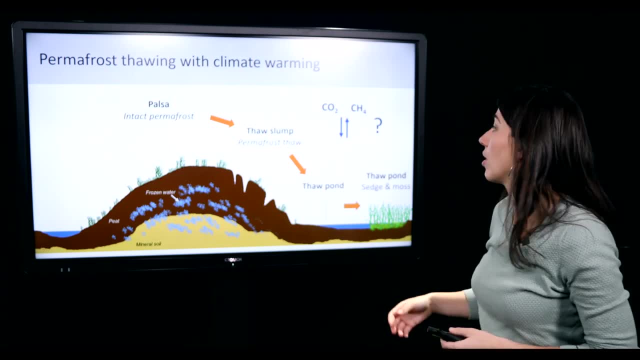 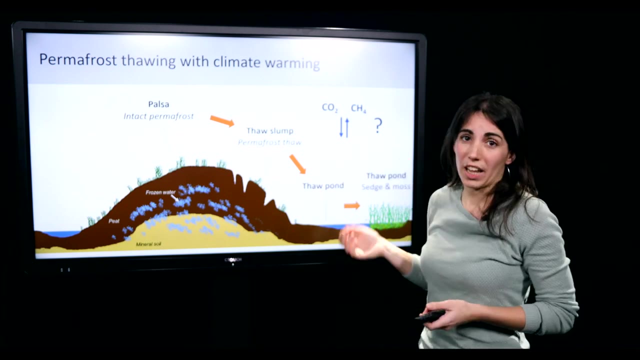 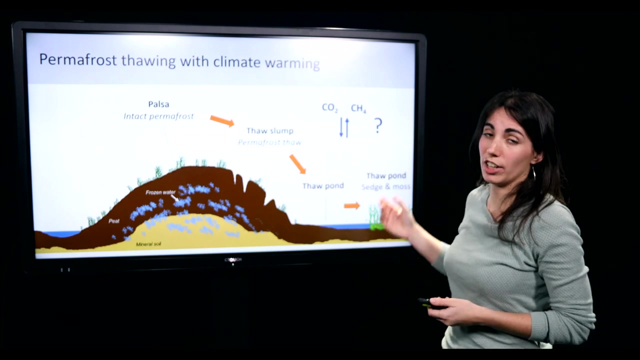 This water is then released to thaw and slump, and also this water is creating thaw ponds. These processes have important consequences for the emission of CO2 and methane, both greenhouse gases. CO2 and methane are greenhouse gases that can enhance warming, and actually methane is a 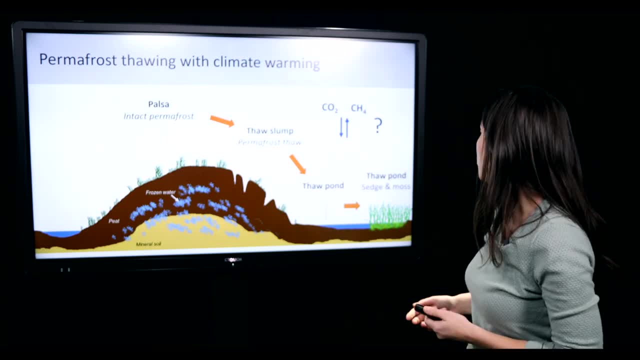 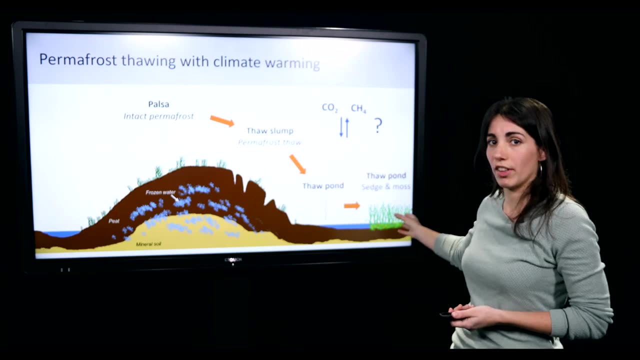 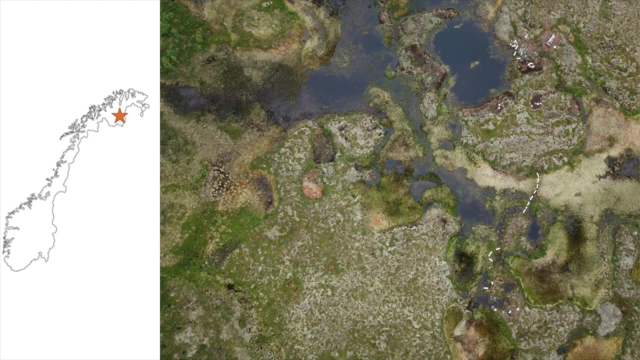 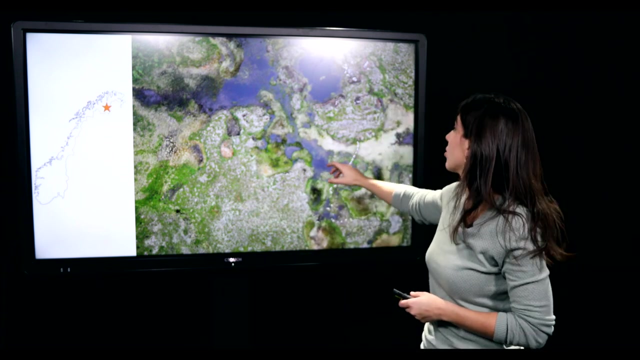 stronger greenhouse gas than CO2.. But when these thaw ponds arise, there can also be regrowth of vegetation and this could also have important effects. This is our research site in northern Norway, where we can see the intact permafrost in these areas, but also the degradation of permafrost which is creating thaw ponds, which is the watery areas. 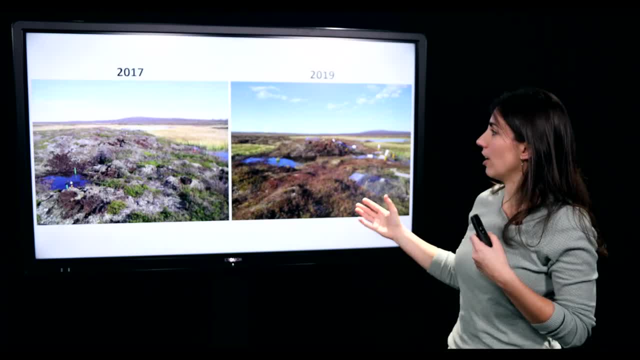 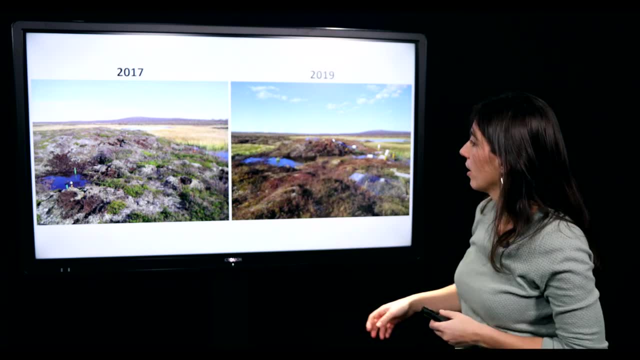 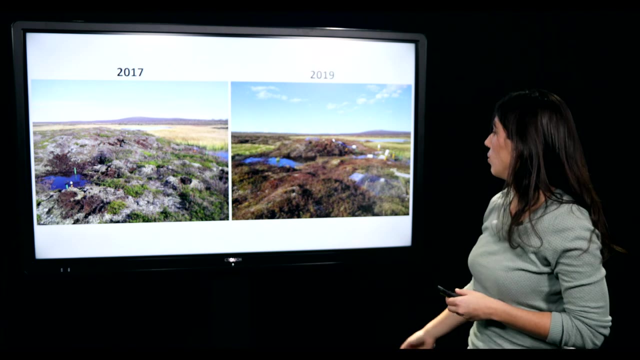 in the picture To have a look at permafrost thaw in our site. here you have a picture in 2017, when we set up the research site, where you can see the permafrost mounds are still nicely intact, while in 2019 we can already see. 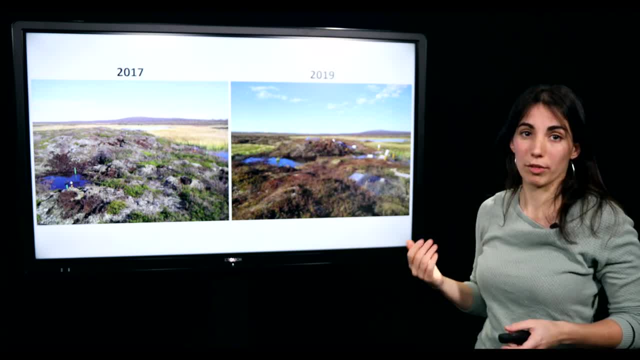 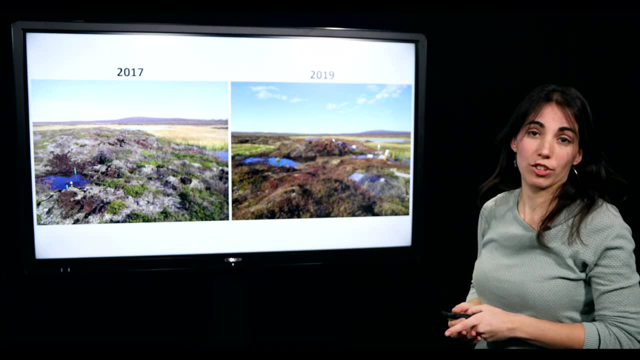 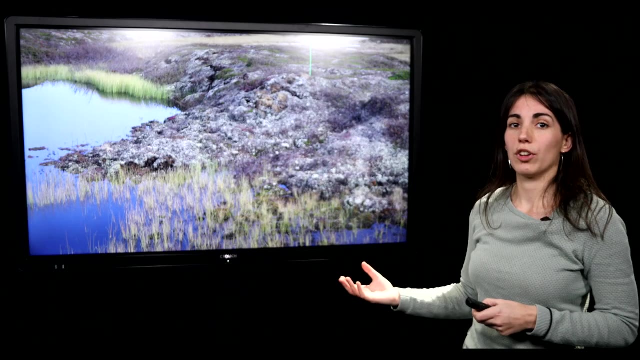 that there is thaw ponds created by permafrost thaw. So this picture indicates that these processes are actually going on in a short amount of time. So we use this hydroponics to create permafrost thaw. We use this hydrological gradient to study, like what happens to the greenhouse gas emissions when